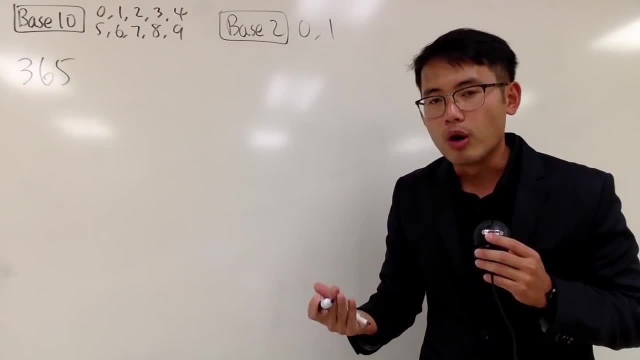 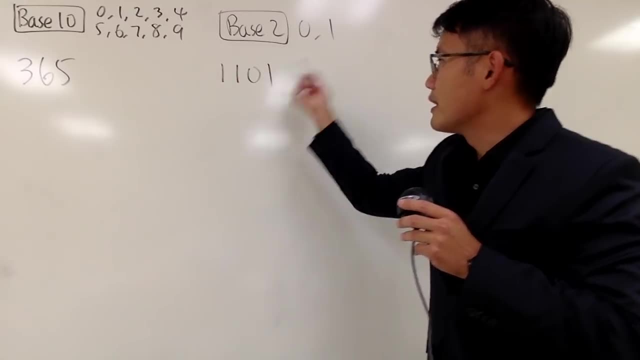 So these are the 2 digits that we can use in the base 2 world to write our number. And let me just write a number for you guys. Maybe let's say 1, 1, 0, 1,, like this: 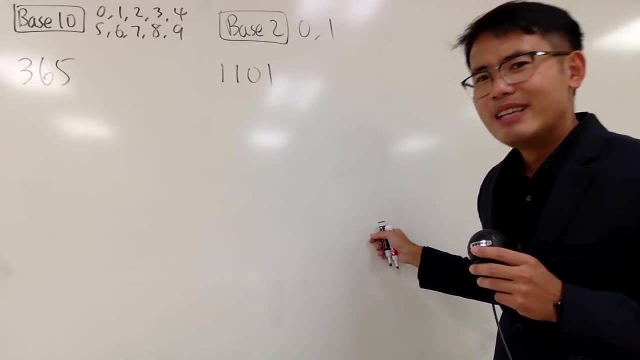 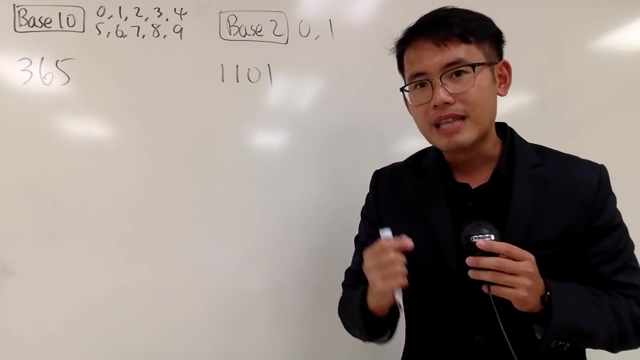 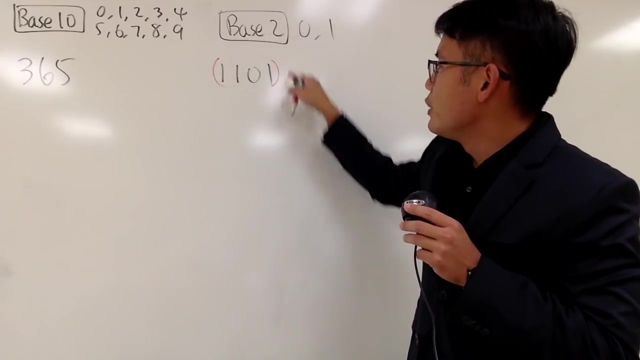 Okay, Hmm, This, and that they look way too alike, But I'm telling you guys that this right here is in base 2.. Now this is how we are going to emphasize that this number is in base 2.. We will put a parenthesis right here and then write the little 2 right here on the bottom right corner to emphasize: this number is in base 2.. 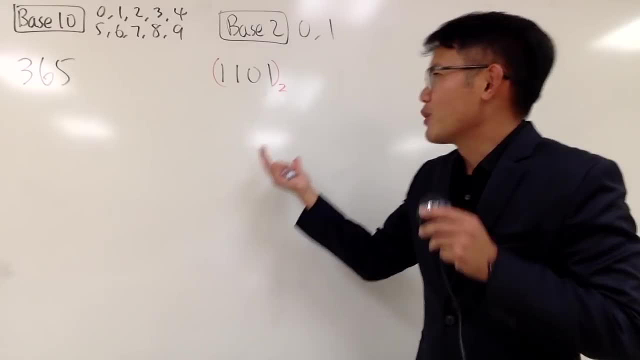 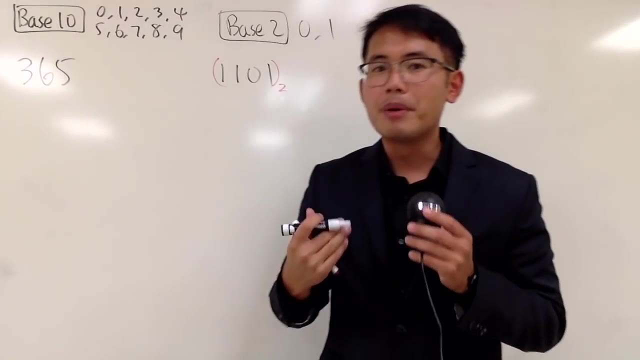 And the next question is: how big is this number then, Like what is its value, right? Well, in order for me to do this, let me come back right here. So let's talk about the expansion of the number 365.. 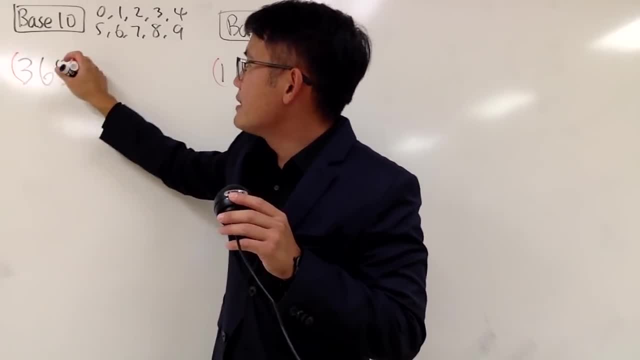 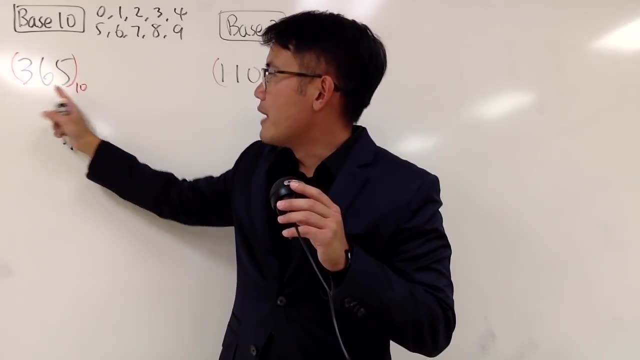 Once again, we are in the base 10.. So I can emphasize that by putting this in the parenthesis, with the little 10 right here, And, as we all know, 365,. the 3 is in the 100th place, the 6 is in the 10th place and the 5 is in the 1st place. 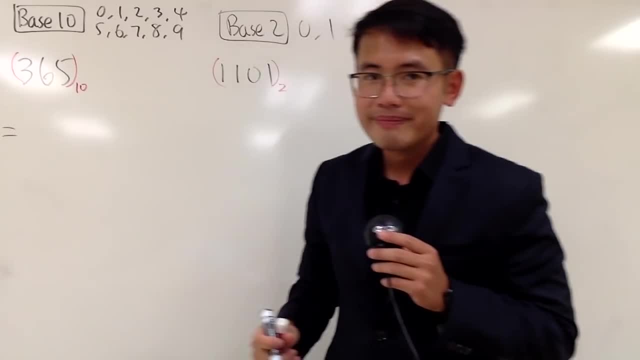 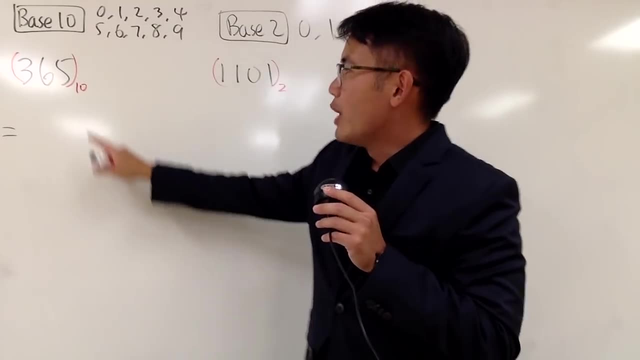 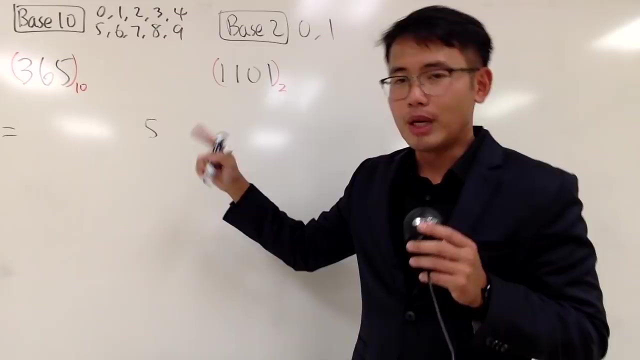 And this is the expansion of this number right, And I usually recommend my students to write this from right to left. Anyway, the 5 is in the 1st place, So let me first write down the 5, and I will multiply by 1, right, because it's in the 1st place. 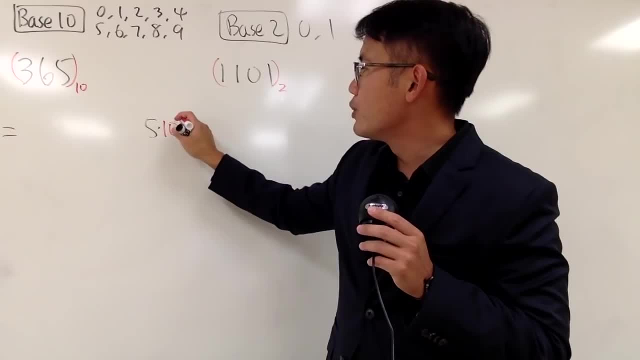 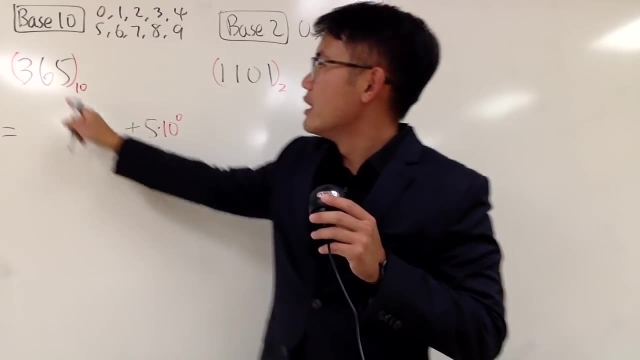 But I will actually write it as times 10 to the 0th power. This is also 1 as well. Now I will add this with 6,, which is in the 10th place, right? So I will just write it as 6.. 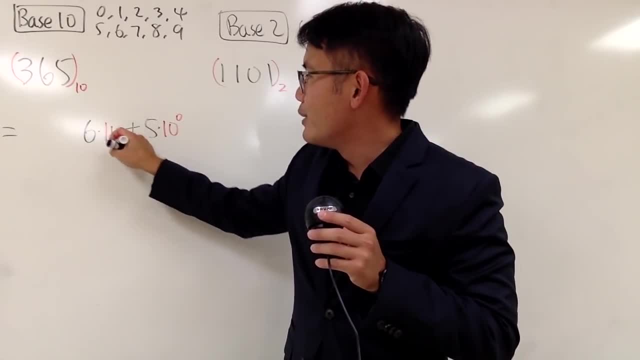 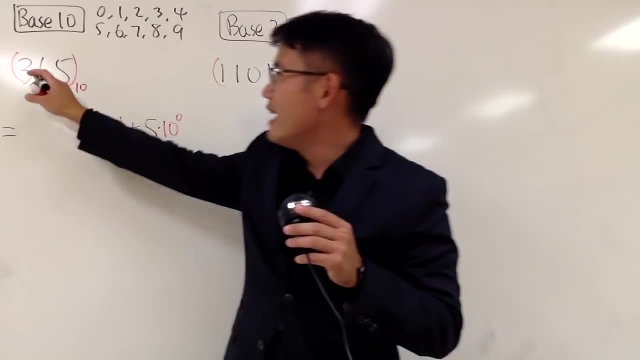 And to emphasize that it's in the 10th place, I will just multiply by 10 to the 1st power And you see this is 10 in the 10th place. Look at that Cool huh. And next, of course, this 3 is in the 100th place. 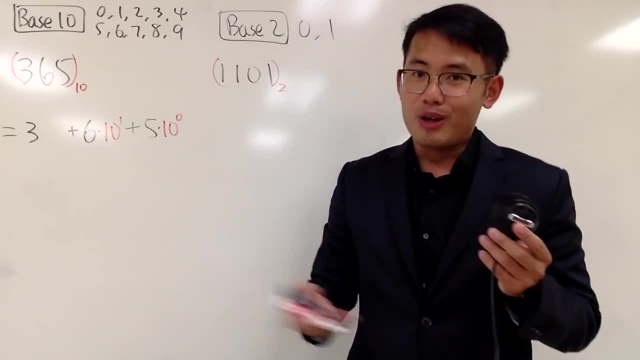 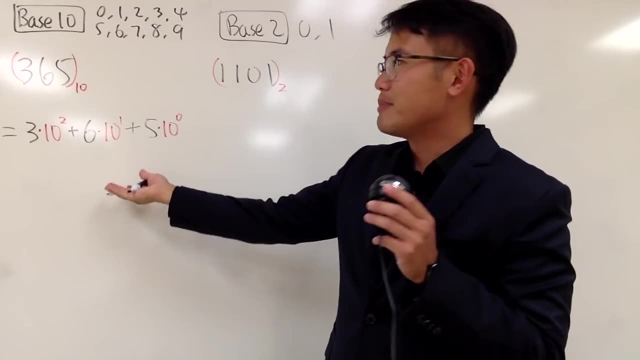 And of course I'm not going to put down: multiply by 100, 1,, 0, 0.. That's too boring. Let's use an exponent: Multiply by 10 to the 2nd power, And this is the expansion for that number. 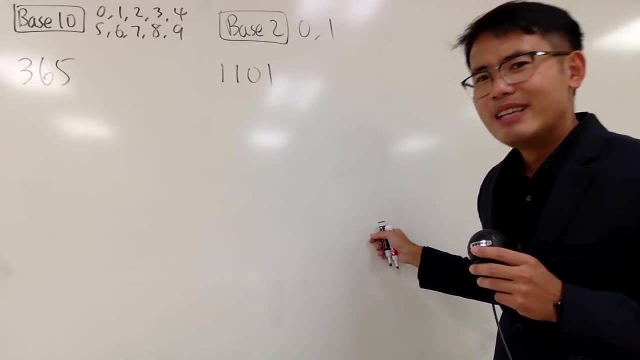 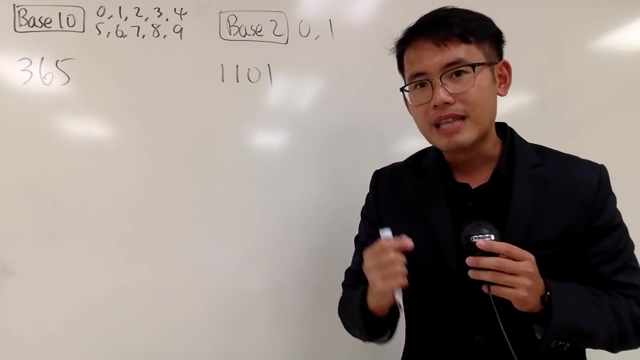 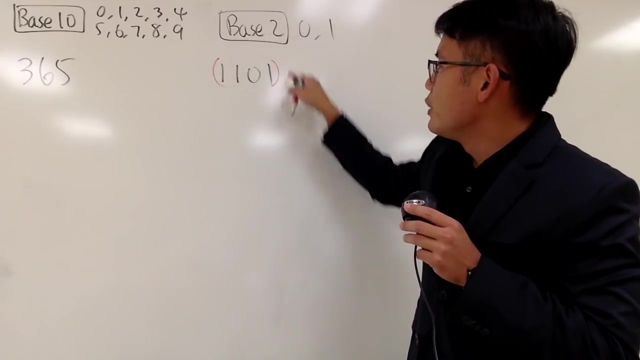 Okay, Hmm, This, and that they look way too alike, But I'm telling you guys that this right here is in base 2.. Now this is how we are going to emphasize that this number is in base 2.. We will put a parenthesis right here and then write the little 2 right here on the bottom right corner to emphasize: this number is in base 2.. 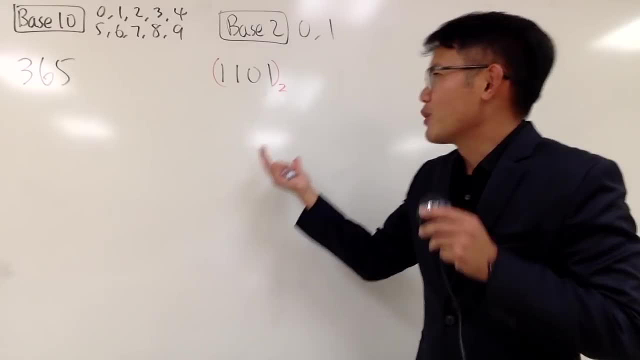 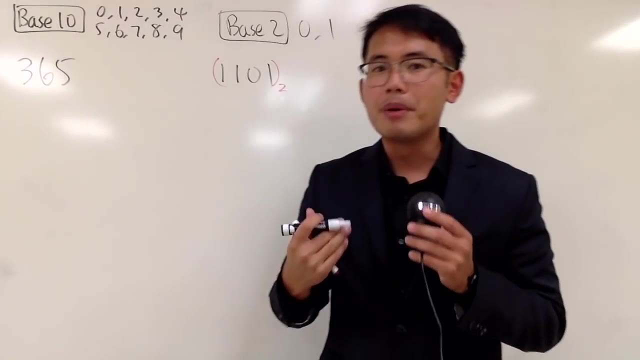 And the next question is: how big is this number then, Like what is its value, right? Well, in order for me to do this, let me come back right here. So let's talk about the expansion of the number 365.. 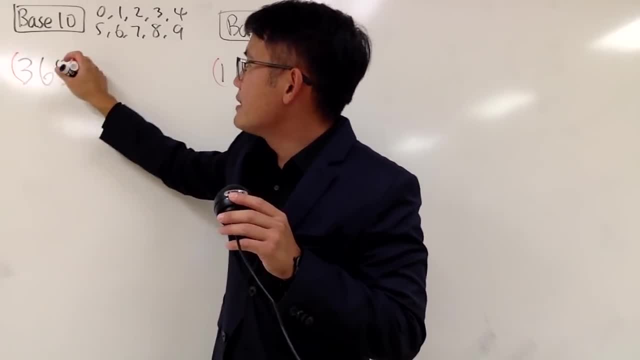 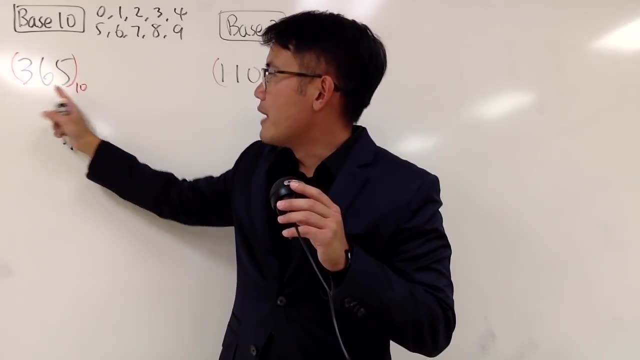 Once again, we are in the base 10.. So I can emphasize that by putting this in the parenthesis, with the little 10 right here, And, as we all know, 365,. the 3 is in the 100th place, the 6 is in the 10th place and the 5 is in the 1st place. 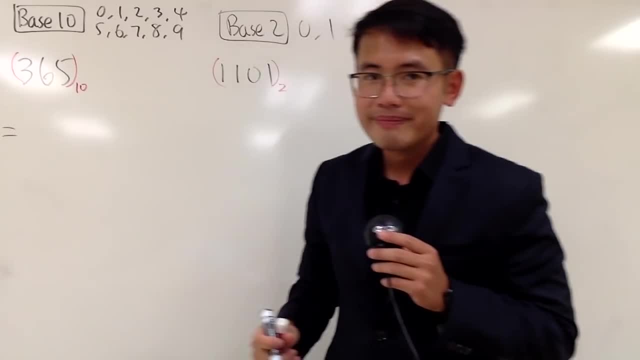 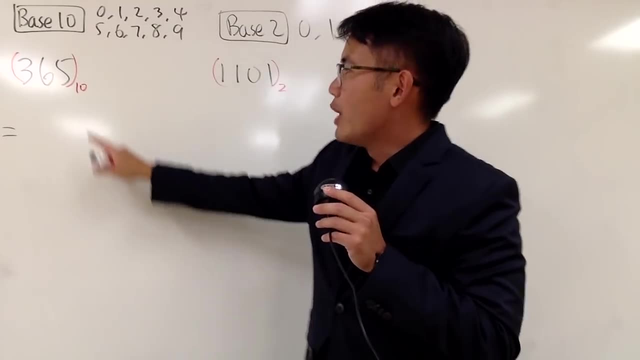 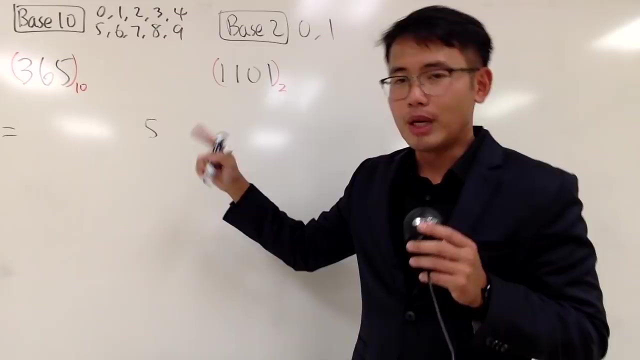 And this is the expansion of this number right, And I usually recommend my students to write this from right to left. Anyway, the 5 is in the 1st place, So let me first write down the 5, and I will multiply by 1, right, because it's in the 1st place. 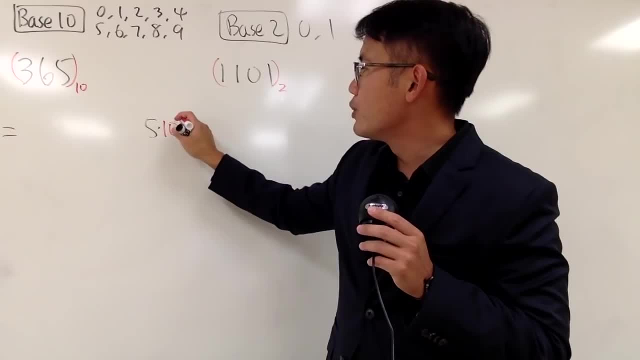 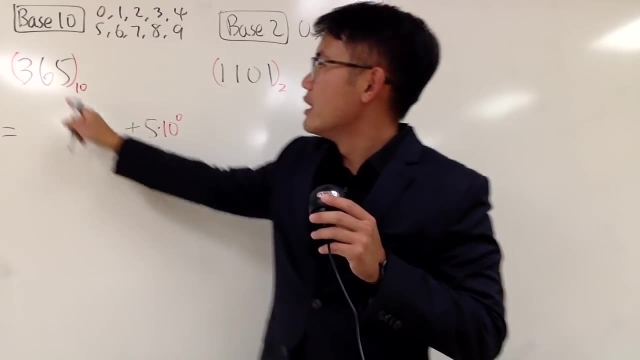 But I will actually write it as times 10 to the 0th power. This is also 1 as well. Now I will add this with 6,, which is in the 10th place, right? So I will just write it as 6.. 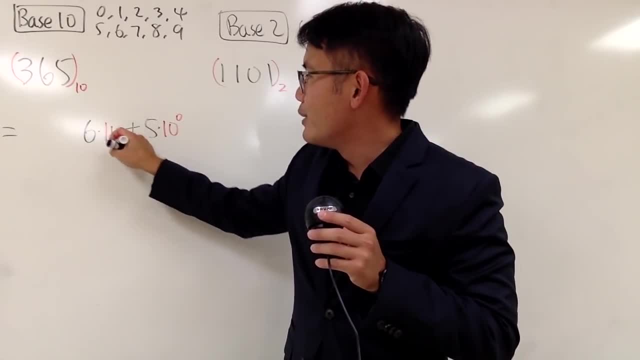 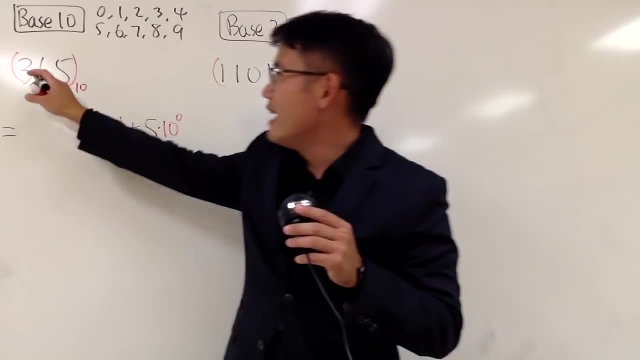 And to emphasize that it's in the 10th place, I will just multiply by 10 to the 1st power And you see this is 10 in the 10th place. Look at that Cool huh. And next, of course, this 3 is in the 100th place. 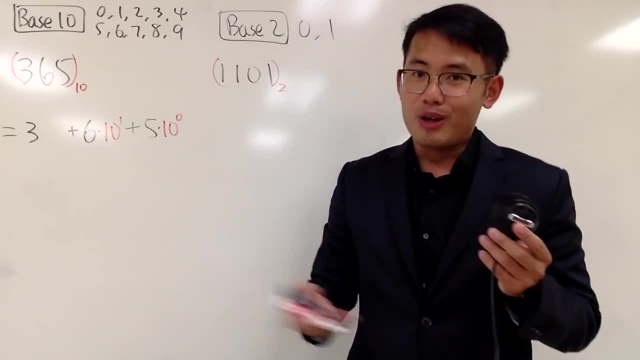 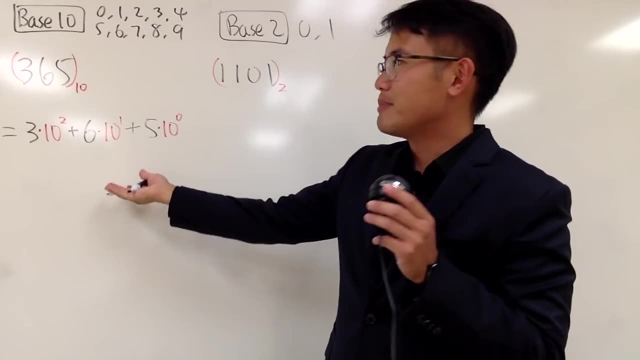 And of course I'm not going to put down multiply by 100, 1,, 0, 0. That's too boring. Let's use exponent Multiply by 10 to the 2nd power, And this is the expansion for that number. 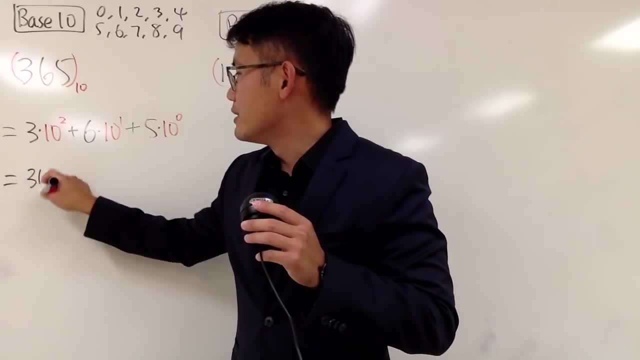 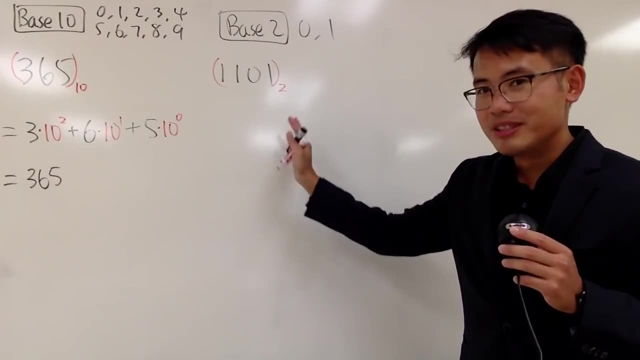 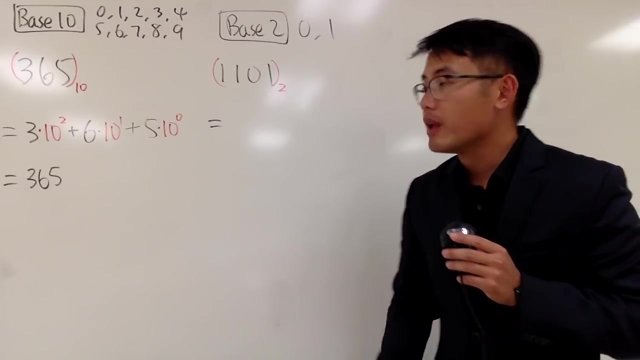 And of course you can work them out. Of course you end up with 365. And that's the value of this. Now, with that being said, you guys will see the connection right here To write the expansion of this, so we can get back to base 10 as well to find out its value. 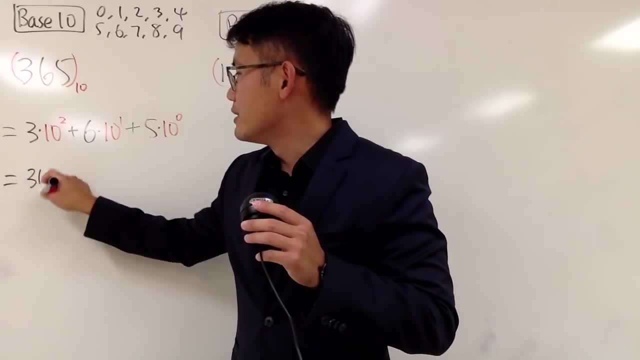 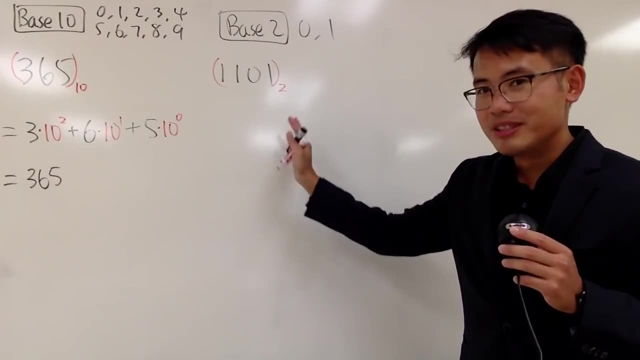 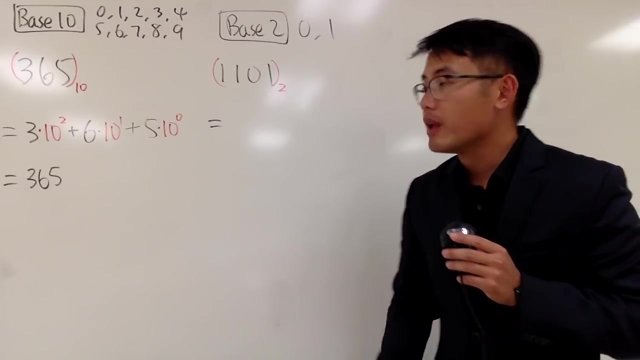 And of course you can work them out. Of course you end up with 365. And that's the value of this. Now, with that being said, you guys will see the connection right here To write the expansion of this, so we can get back to base 10 as well to find out its value. 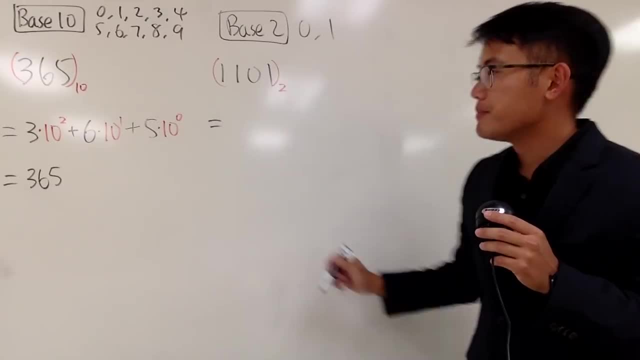 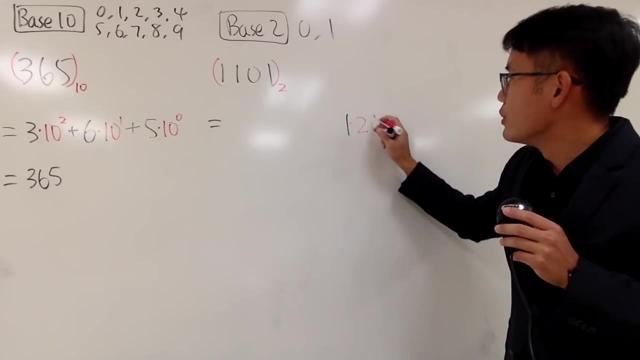 I will begin with the first digit right here from the right. This is a 1,, so write down 1.. And this time I will multiply by 2 to the 0th power, because we're talking about base 2.. 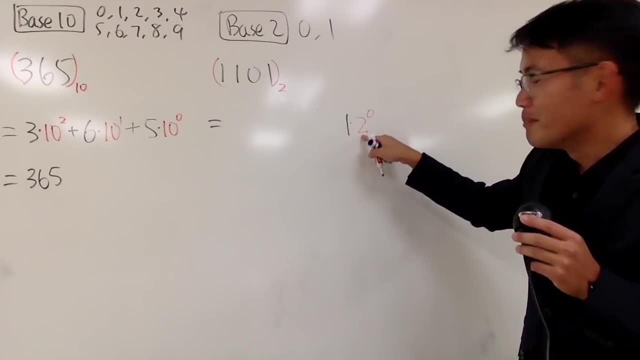 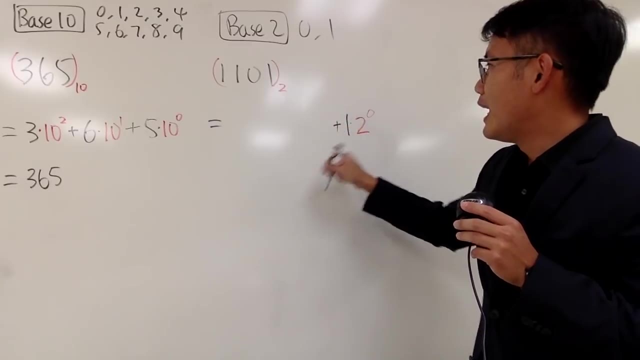 And you see this also. this is also the base for the exponent right. We have 2 to the 0th power, like that. Next, I will just add the- we have 0 right here and multiply by 2 to the 1st power. 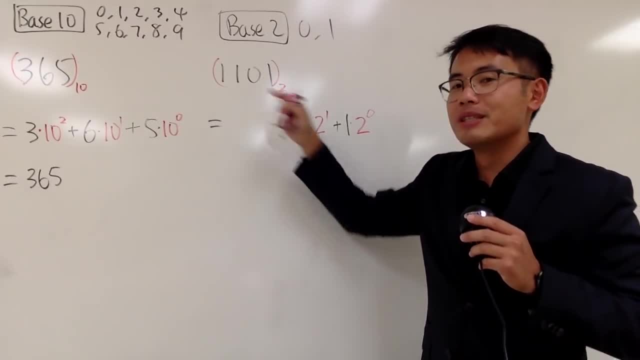 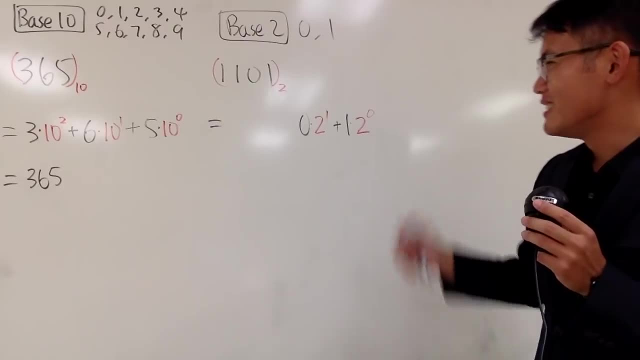 because technically I will say this is 2 to the 1st power place. Likewise, this right here was 10 to the 1st place, namely the 10th right, Similar, And now you pretty much just do the rest. 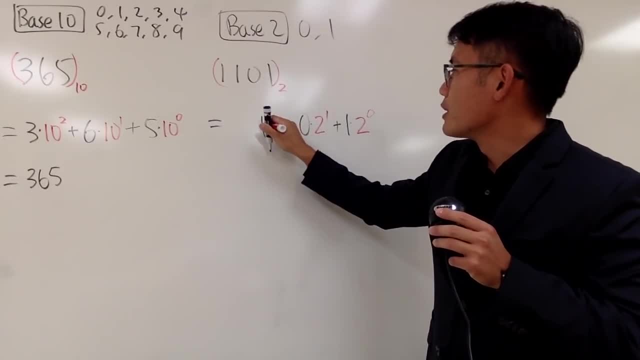 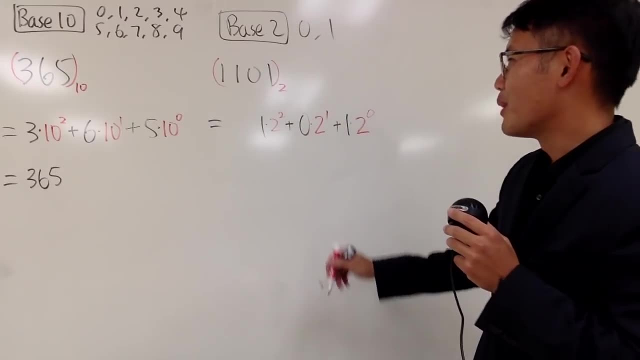 Next we have 1, and I will multiply by 2 to the 2nd power. You just build up the power right: 0,, 1,, 2, and so on. Continue the power. Lastly, right here, we have 1 times 2 to the 3rd power. 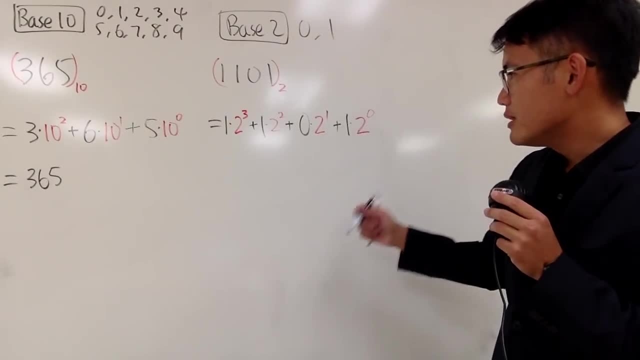 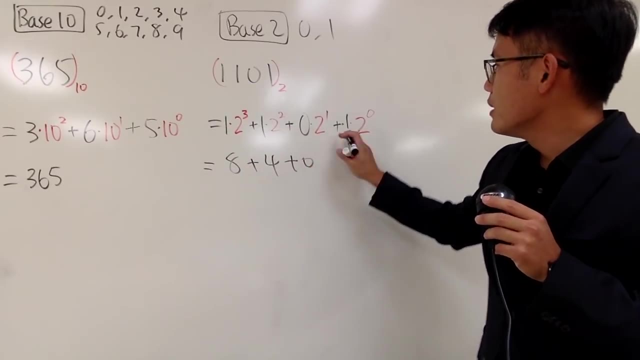 And then, of course, in the end we just add them up. Now, this is just a word of operation question. Let's see, this is 8,, this is 4,, this is 0, and this is 1.. 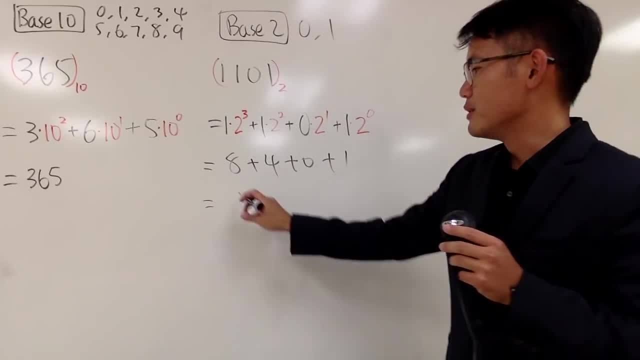 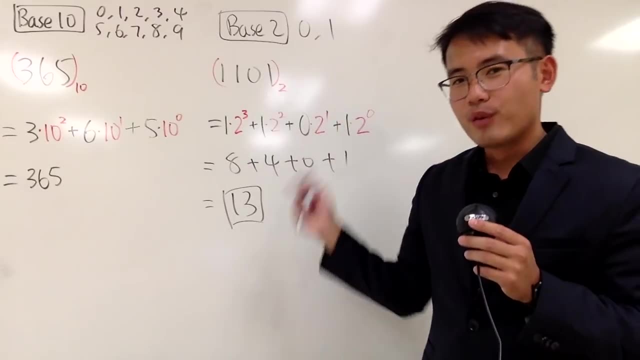 And, of course, you add them up. The answer to this is 13,, and that's pretty much it. So, as you guys can see, 1, 1, 0, 1 in base 2 is, of course, smaller than 365 in base 10,. 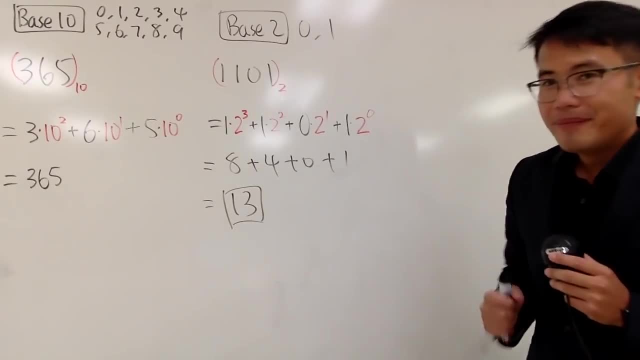 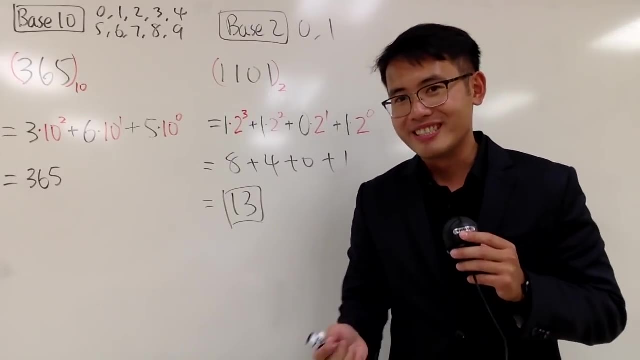 because this right here, the value is only 13.. Okay, now let me give you guys another digit to use And, by the way, in fact, you can talk about base whatever you want. Let me just give you guys another digit to use. so we are talking about base 3.. 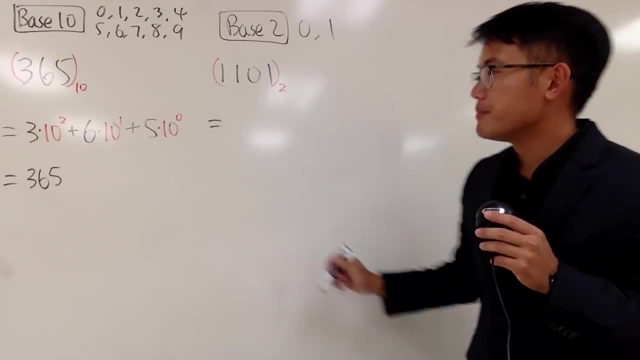 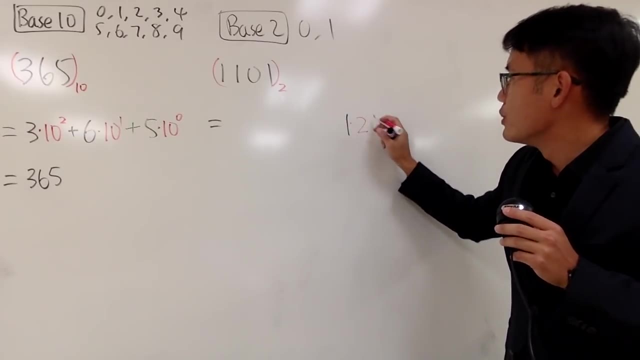 I will begin with the first digit right here from the right. This is a 1,, so write down 1.. And this time I will multiply by 2 to the 0th power, Because we're talking about base 2.. 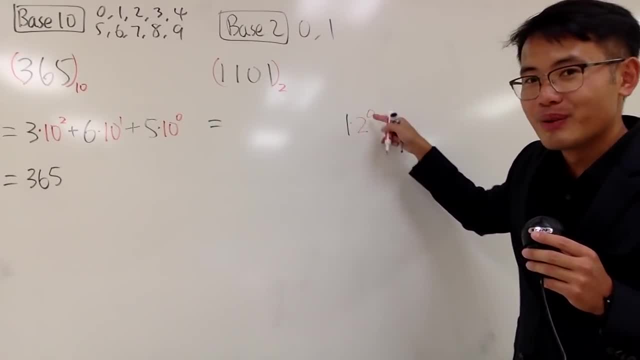 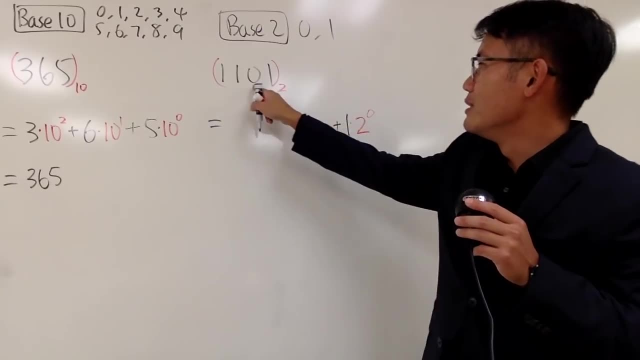 And you see this also. this is also the base for the exponent right. We have 2 to the 0th power, like that. Next, I will just add the- we have 0 right here and multiply by 2 to the 1st power. 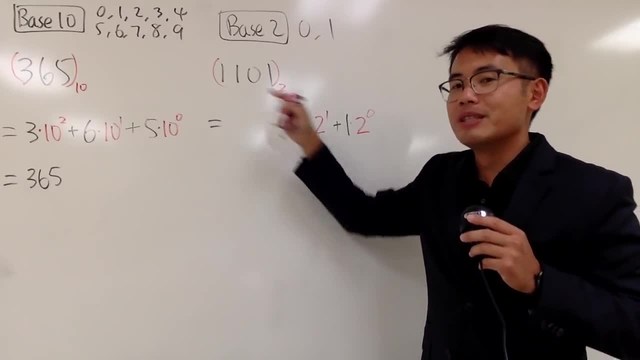 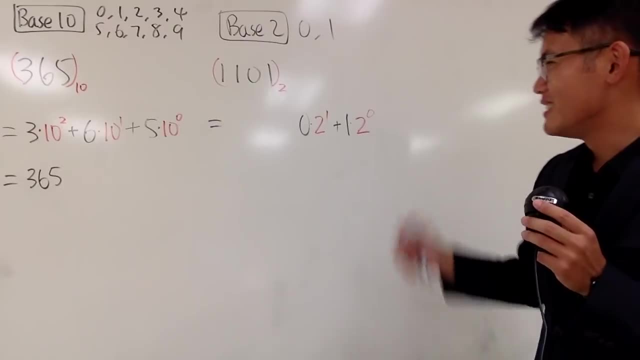 Because technically I will say this is 2 to the 1st power place. Likewise, this right here was 10 to the 1st place, namely the 10th right, Similar, And now you pretty much just do the rest. 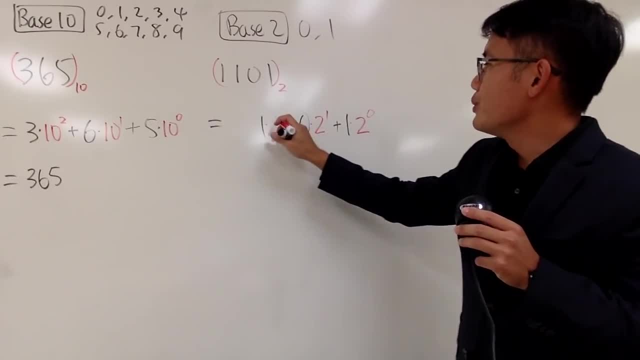 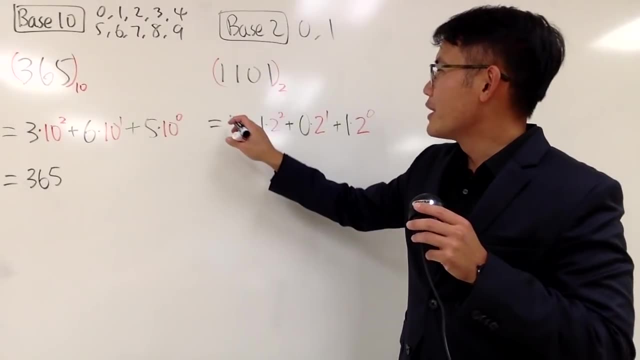 Next we have 1, and I will multiply by 2 to the 2nd power. You just build up the power right: 0,, 1,, 2, and so on. Continue the power. Lastly, right here, we have 1 times 2 to the 3rd power. 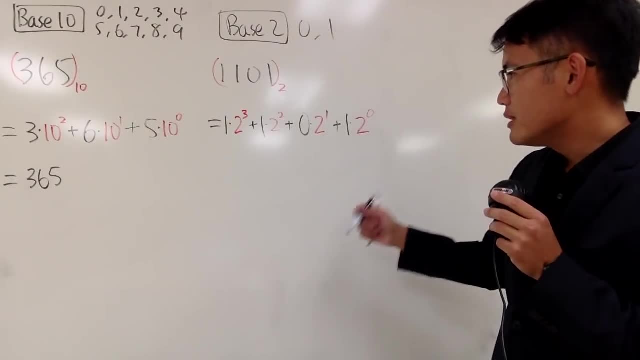 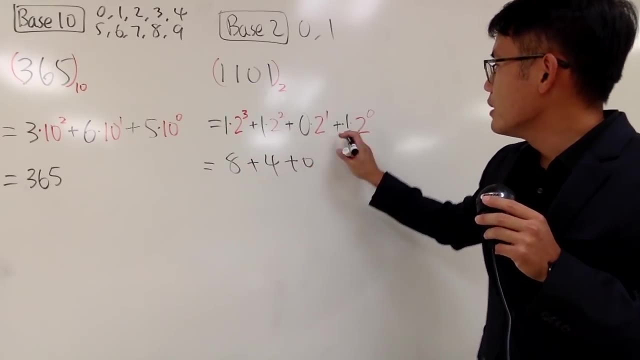 And then, of course, in the end we just add them up. Now, this is just a word of operation question. Let's see, this is 8,, this is 4,, this is 0, and this is 1.. 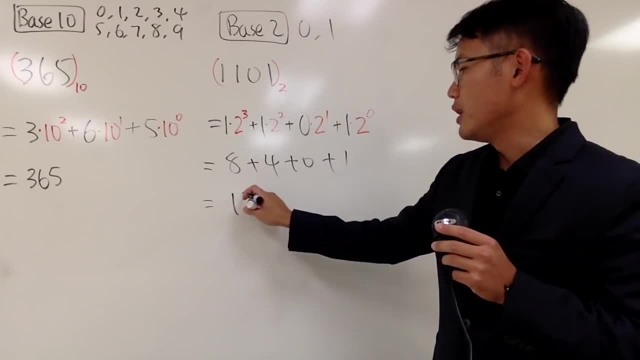 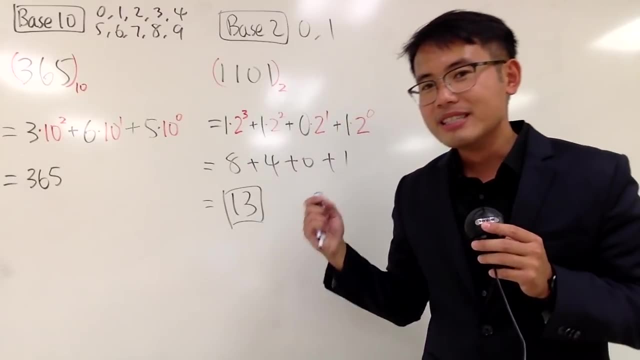 And, of course, you add them up. The answer to this is 13. And that's pretty much it. So, as you guys can see, 1, 1, 0, 1 in base 2 is, of course, smaller than 365 in base 10.. 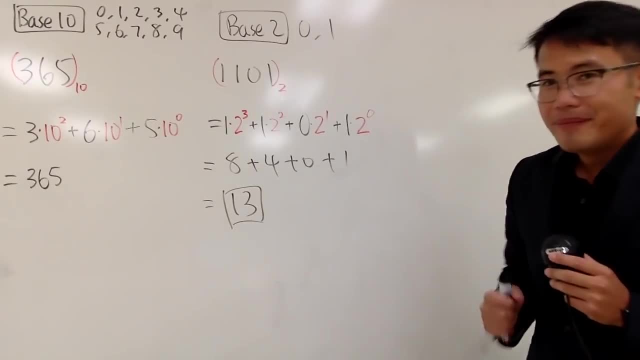 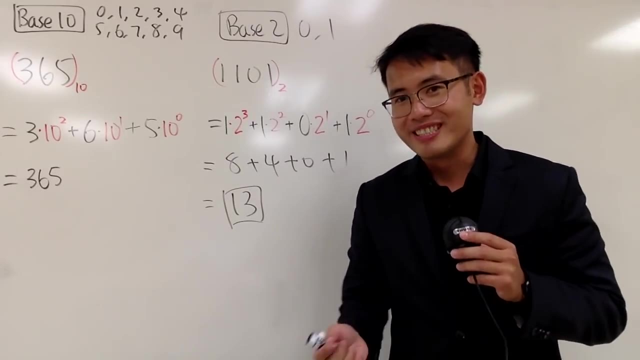 Because this right here, the value is only 13.. Okay, now let me give you guys another digit to use And, by the way, in fact, you can talk about base, whatever you want. Let me just give you guys another digit to use. 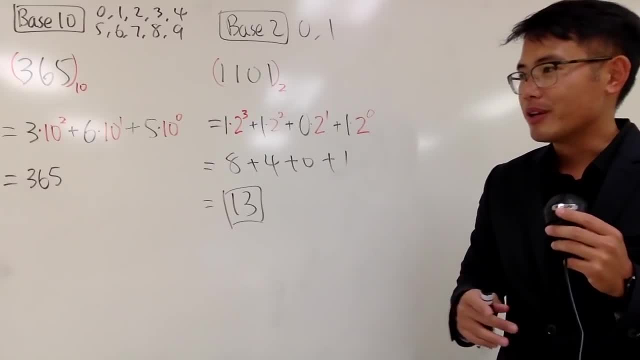 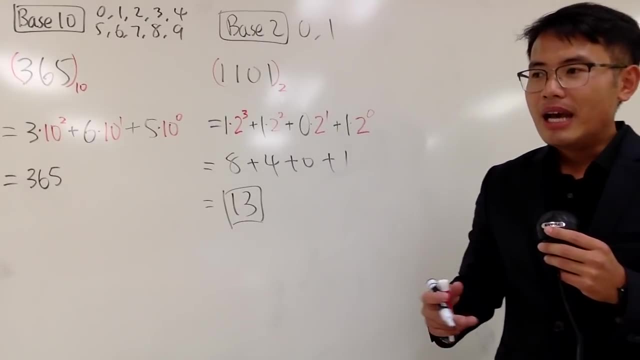 So we are talking about base 3. But technically you can talk about base 8,, base 10 already, base 12, base 16,, base 32.. And you might be wondering: okay, we only have 10 digits normally, right? 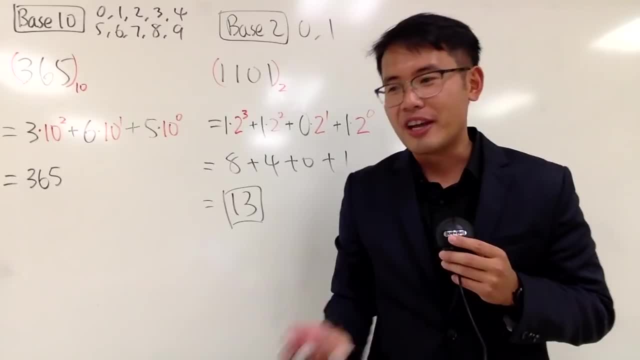 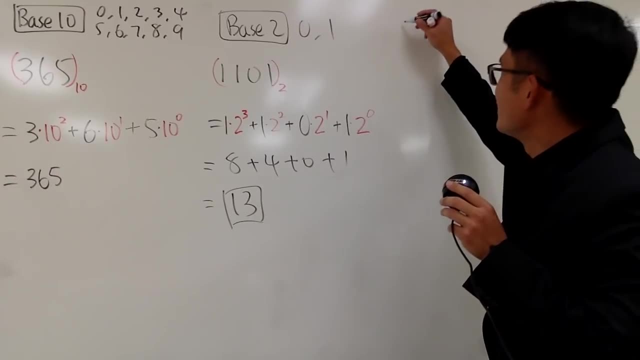 How can we do base 16?? In that case, you can use Chinese data. No, just kidding. You can use English alphabet like A, B, C, D. Anyway, I'm not going to work that out, I'm just going to do base 3, right. 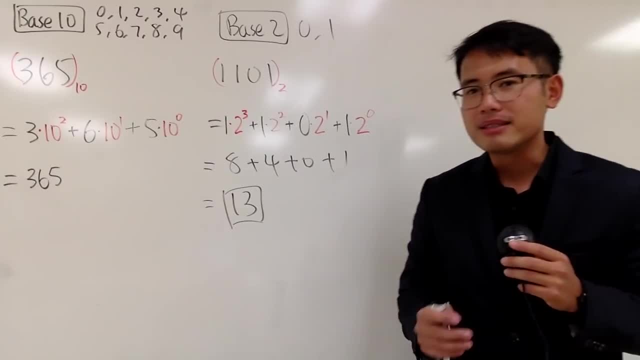 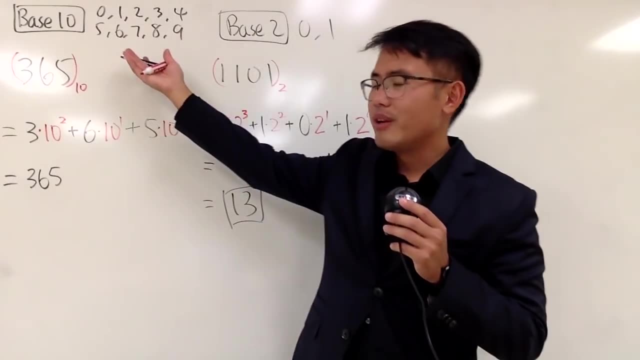 But technically you can talk about base 8, base 10 already, base 12, base 16,, base 32.. And you might be wondering: okay, we only have 10 digits normally, right? How can we do base 16?? 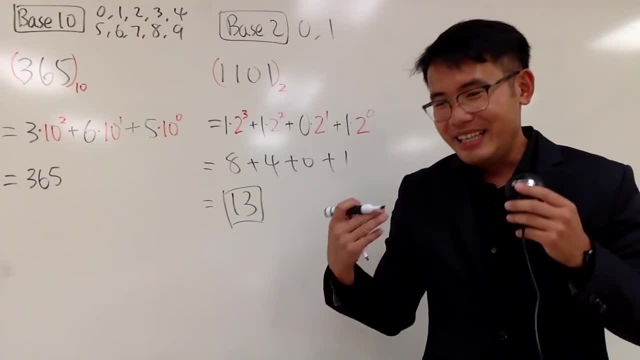 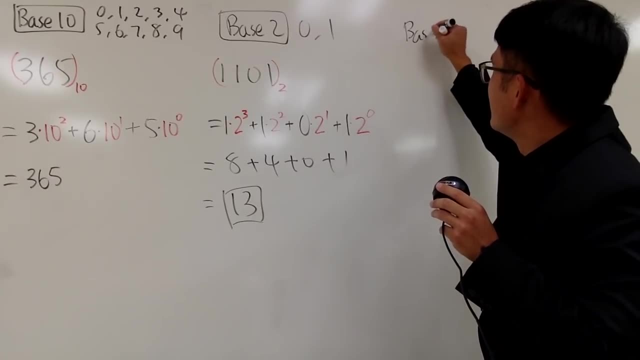 In that case, you can use Chinese data. No, just kidding. You can use English alphabet, ABCD. Anyway, I'm not going to work that out, I'm just going to do base 3.. Right, And for base 3,. 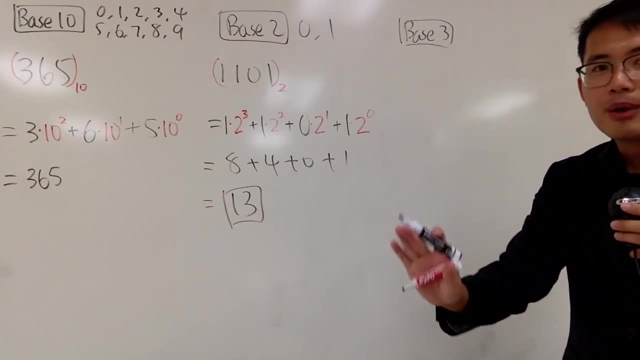 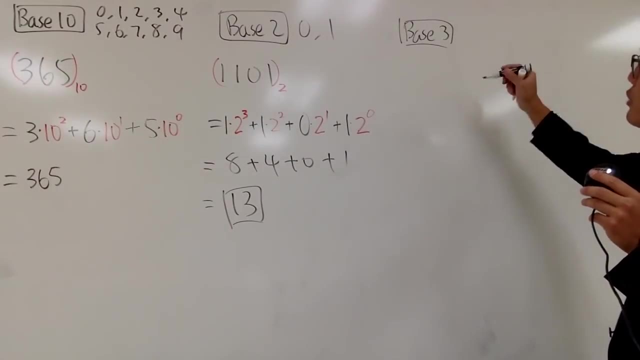 I have one more digit to use, so I'm going to just have another digit. So let me just use the next one, of course, 2.. So in the base 3 world I have 0,, 1, and 2 to be used. 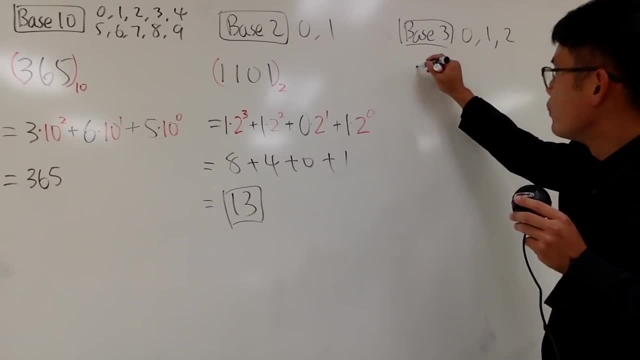 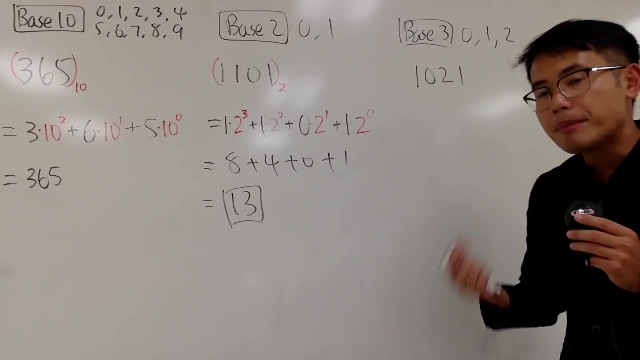 And let me just give you guys a quick example. Suppose I have 1,, 0,, 2,, 1, like this. You see, I can use 0,, 1, or 2 to write my number in base 3.. 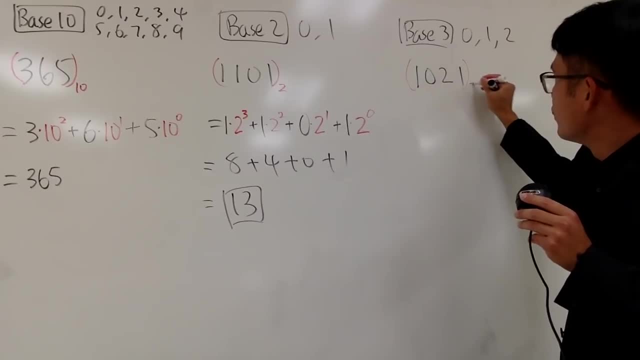 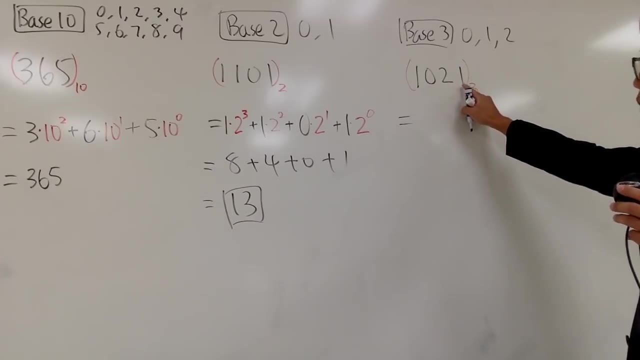 And I will emphasize this is base 3, so I'll put apprentices With the little 3 right here And now let's figure out the value of this Once again, starting from the number right here, from the right, This is: I have 1 right here. 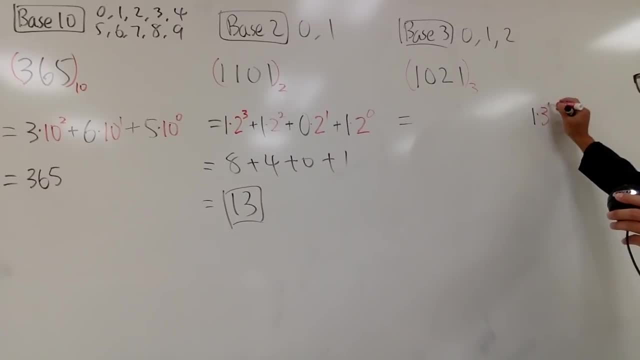 And I multiply it by 3 for the base: 2 to the 0th power. Next I can use 2.. And I multiply it by 3 to the 1st power And the next. I have 0.. 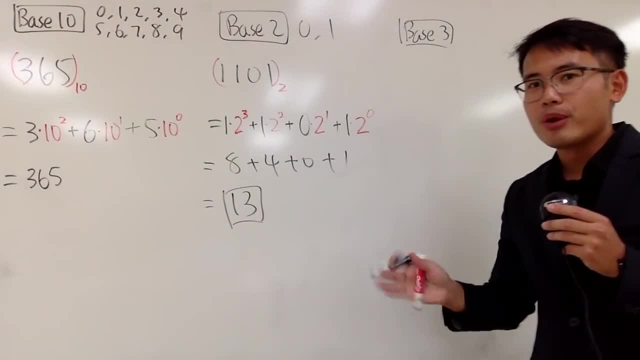 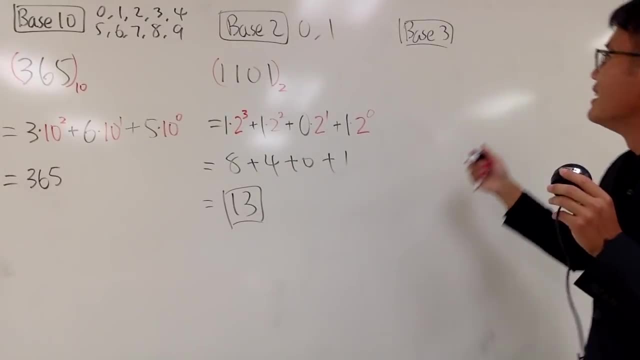 And for base 3, I have one more digit to use, So I'm going to just have another digit. So let me just use the next one, of course, 2.. So in the base 3 world I have 0,, 1, and 2 to be used. 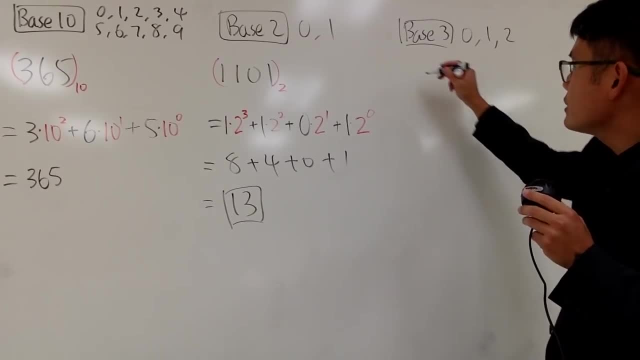 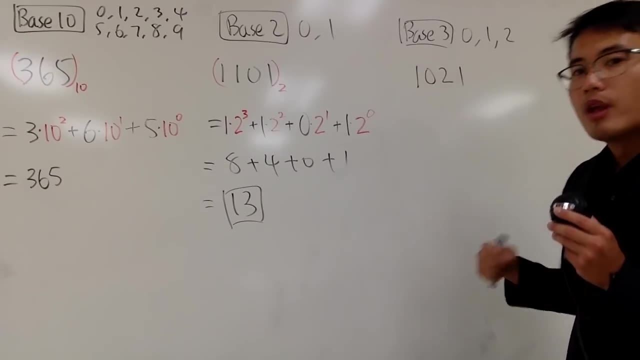 And let me just give you guys a quick example. Suppose I have 1,, 0,, 2,, 1, like this. You see, I can use 0,, 1, or 2 to write my number in base 3.. 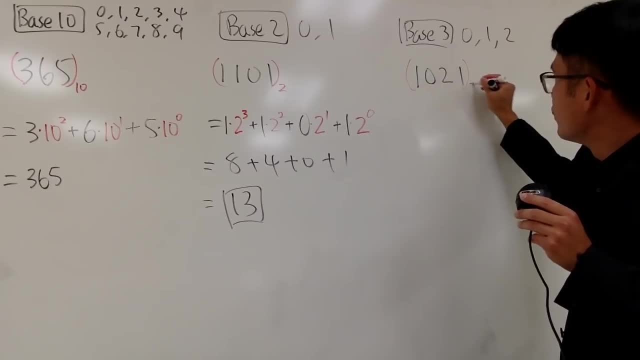 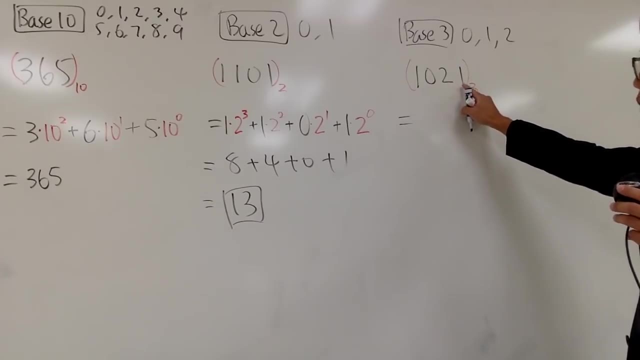 And I will emphasize this is base 3.. So I'll put a parentheses with a little 3 right here And now let's figure out the value of this Once again, starting from the number right here, from the right, This is: I have 1 right here. 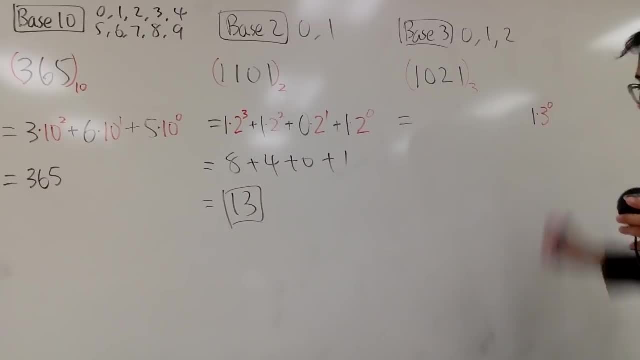 And I multiply it by 3 for the base to the 0th power. Next I can use 2.. And then I multiply by 3 to the first power And then next I have 0.. I multiply by 3 to the second power. 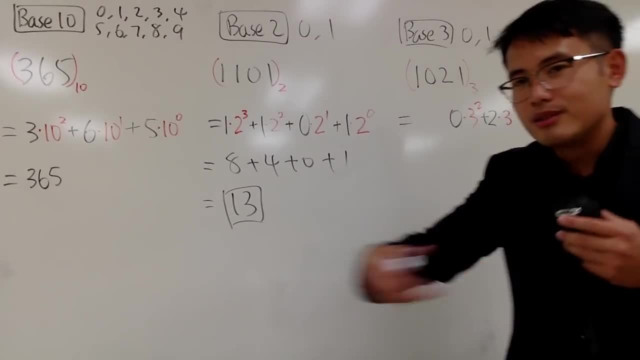 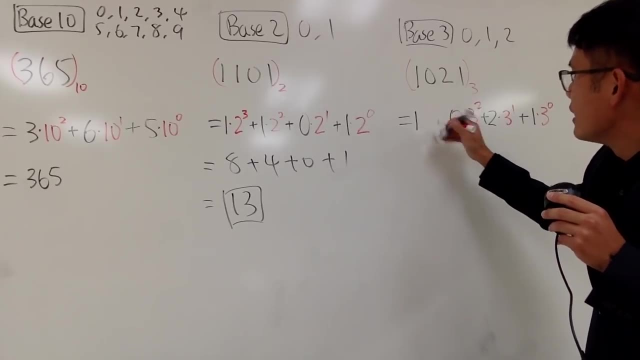 And, of course, you can have the digit as long as you want, right, But I just want to do this and you guys will see the pattern. Anyway, the last one that I have is 1 times 3 to the third. 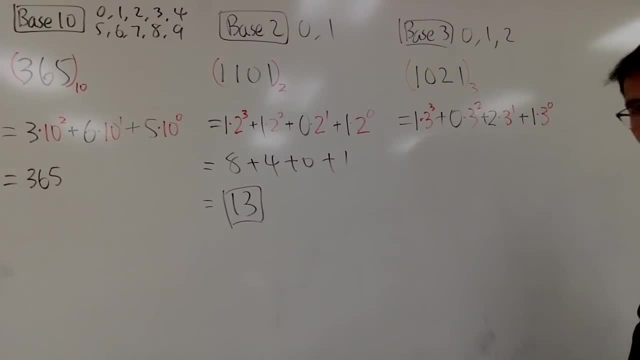 And then, of course, I just have to add them up. Now, this is 27, and 0 times this is just 0. And this is pretty much 2 times 2,, which is 6.. And this is 1.. 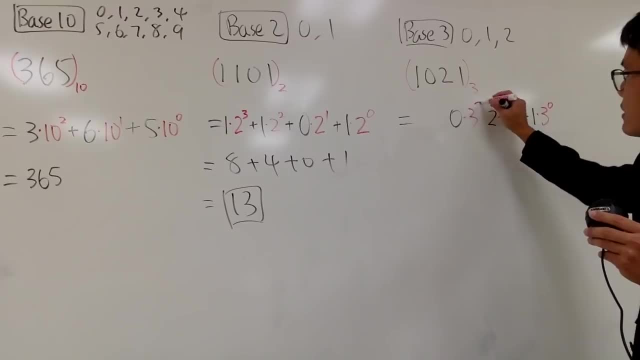 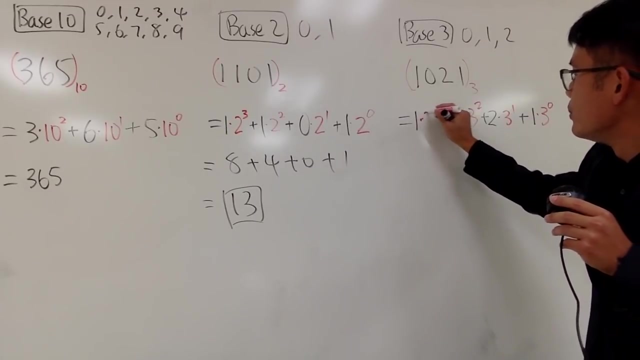 I multiply it by 3.. 3 to the 2nd power And of course you can have the digit as long as you want, right? But I just want to do this and you guys will see the pattern. Anyway, the last one that I have is 1 times 3 to the 3rd. 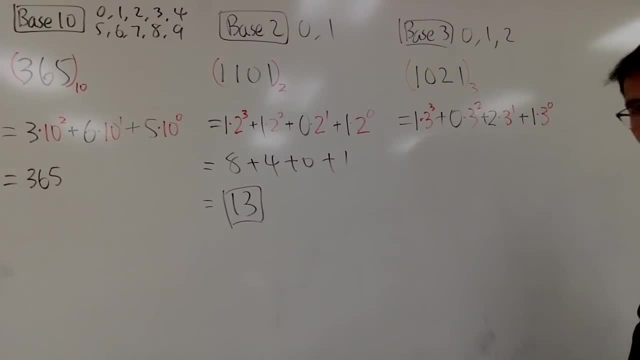 And then, of course, I just have to add them up. Now, this is 27, and 0 times this is just 0. And this is pretty much 2 times 2,, which is 6.. And this is 1.. 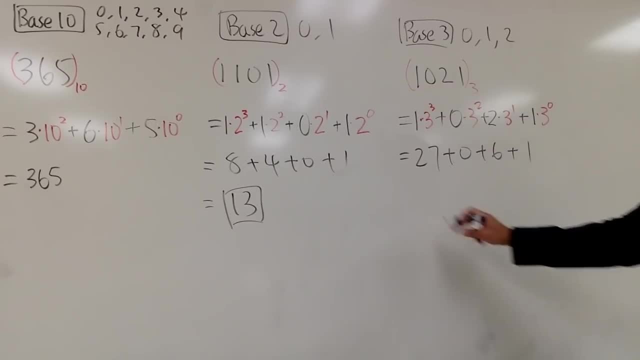 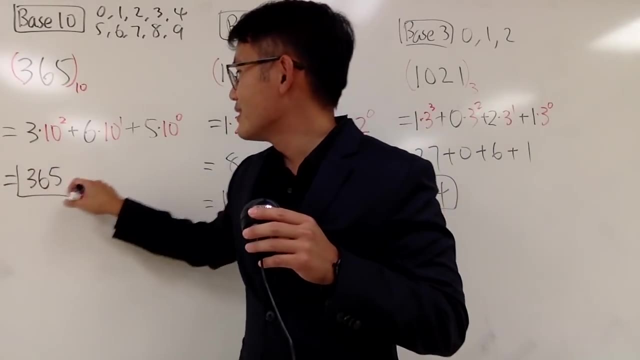 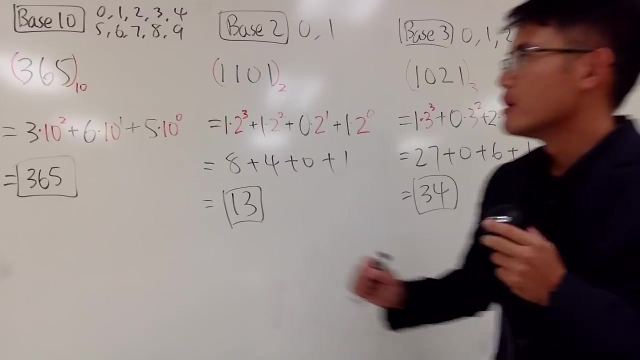 So this plus that is 33, plus 1 is 34.. So this right here it has the value 34,, right? So of course this is pretty much it. And perhaps the next question is what happens if you start with a base 10 number? 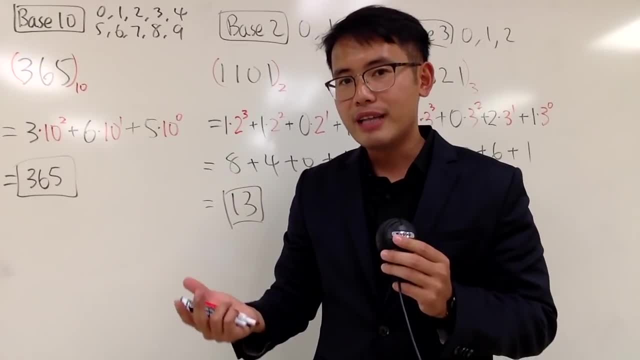 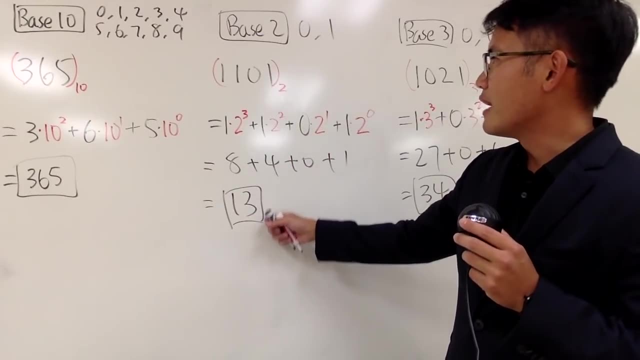 let's say you have the value 365? How can you convert that Into a base 2 number? Likewise, how can we go backward, Starting from 13,? how can I write it as 1 1 0, 1 in base 2?? 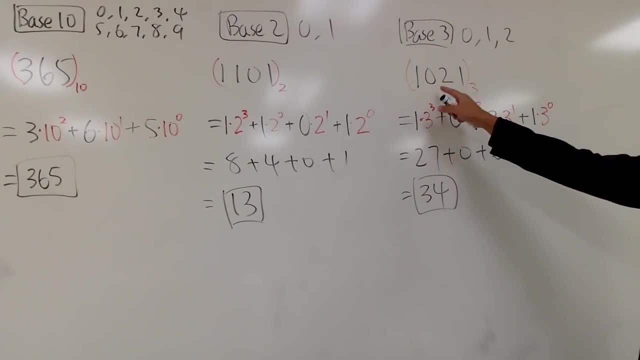 Or if I start with 34, how can I write it as 1, 0, 2, 1 in base 3?? And I will just work that out for you guys in the next video. for that,